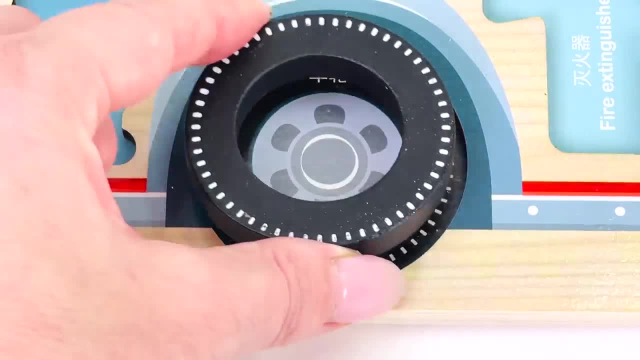 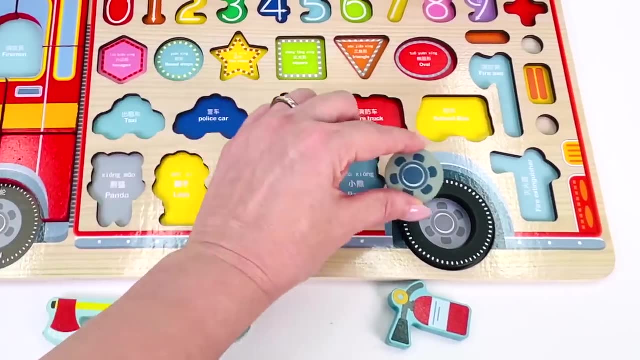 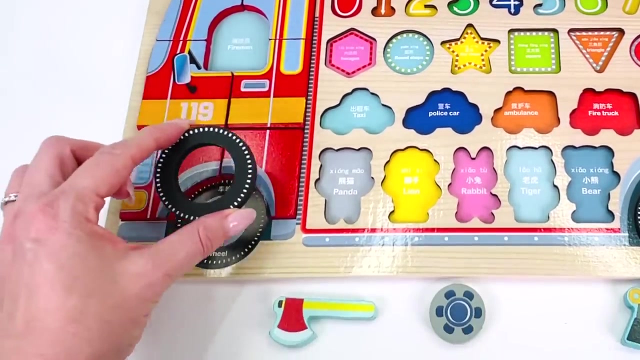 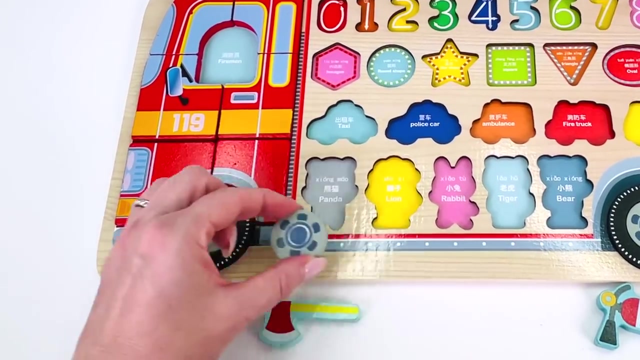 like a tire. I think it will go here. Yes, on the wheel, And how about this one? This little circle is the hubcap, And I think we'll need another wheel. We'll place it right here And find the other hubcap and place it in the middle of the tire. 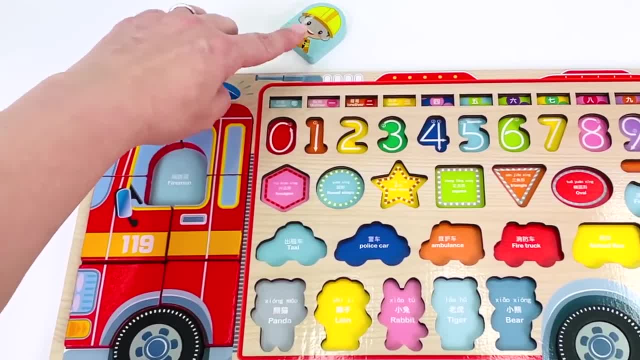 Great job, Oh, and don't forget the fire person. We'll put you here. Great job, Oh, and don't forget the fire person. We'll put you here. Great job, Oh, and don't forget the fire person. We'll put you. 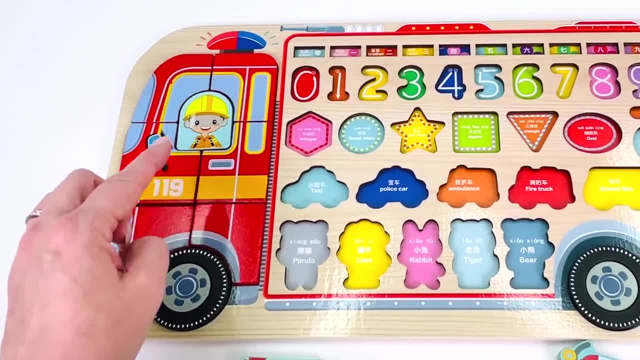 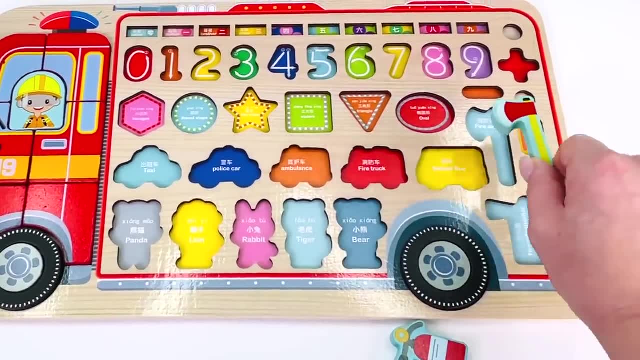 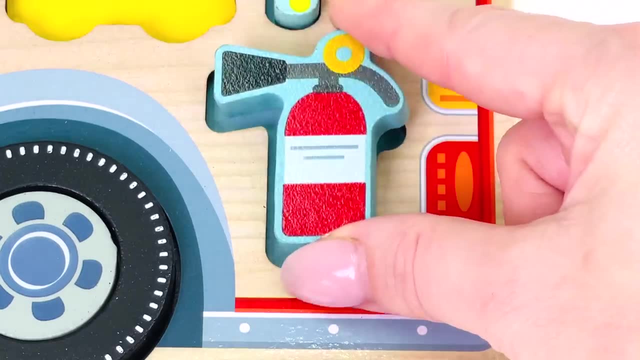 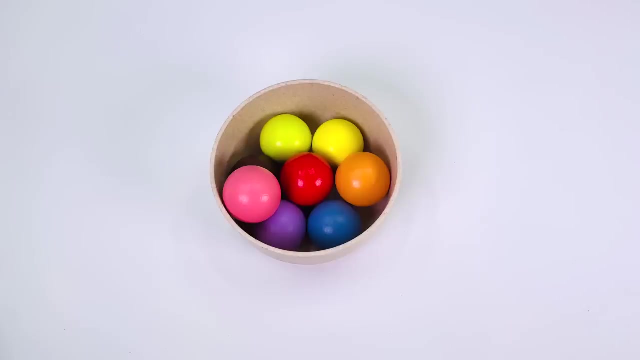 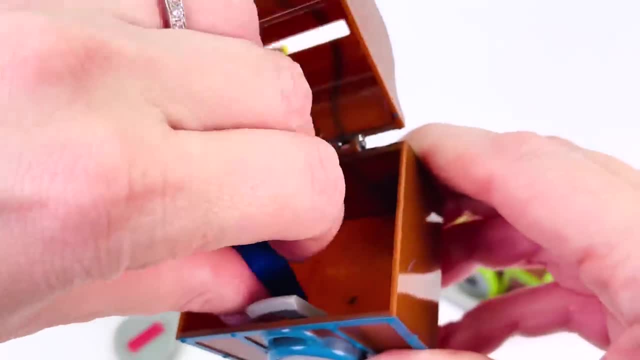 put you here: Great job. Oh, and don't forget the fire person. We'll put you here: Great job. Oh, and don't forget the fire person. We'll put you here. Great job. Let's open this one, Oh, and. 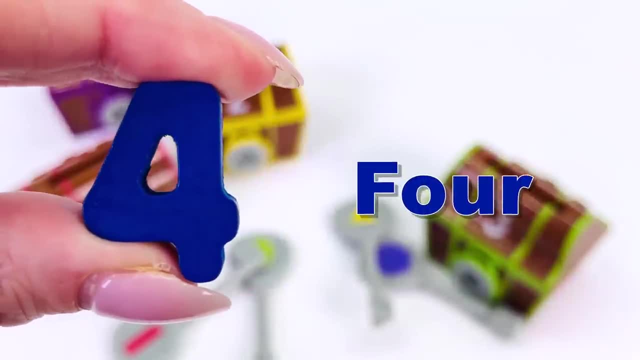 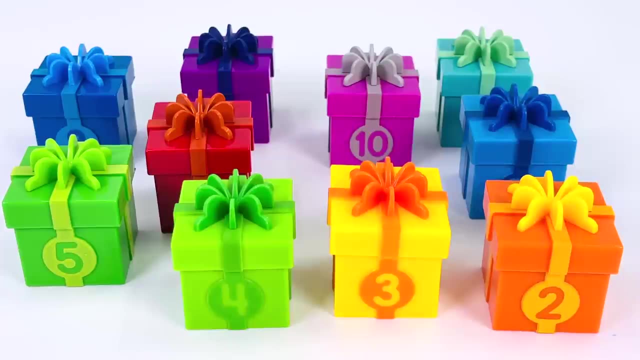 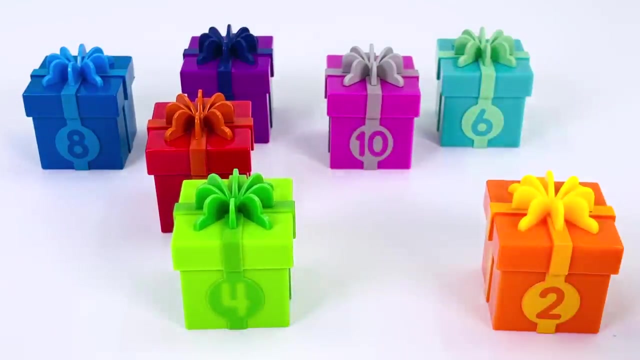 don't forget the fire person. We'll that. We found another number. We found another number. We found another number, The number four. We found another number, The number four. Let's put it back in the puzzle: The number four. 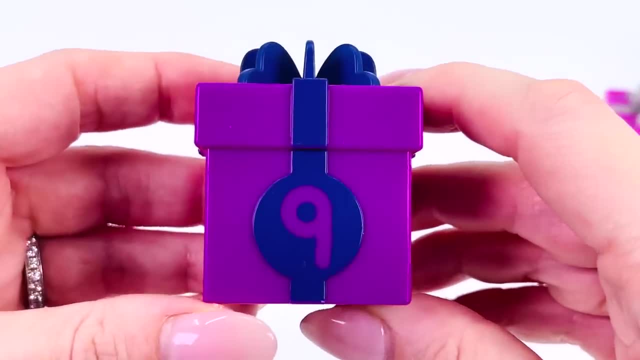 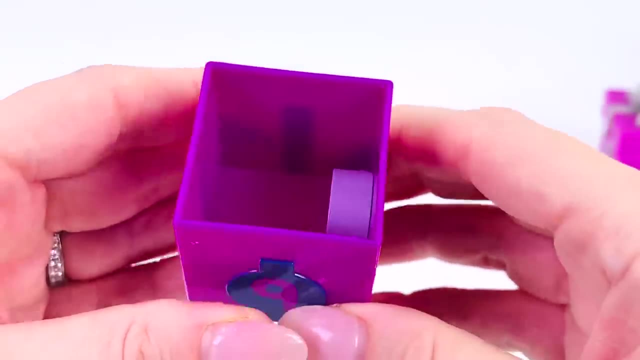 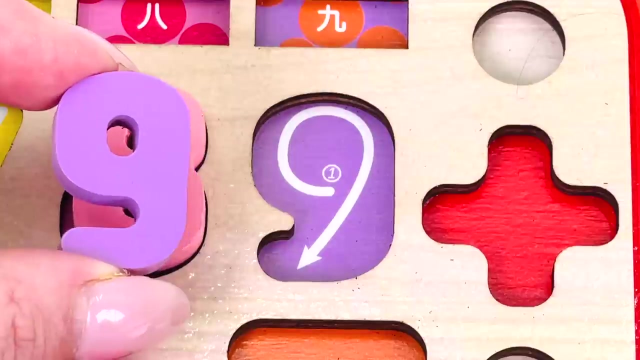 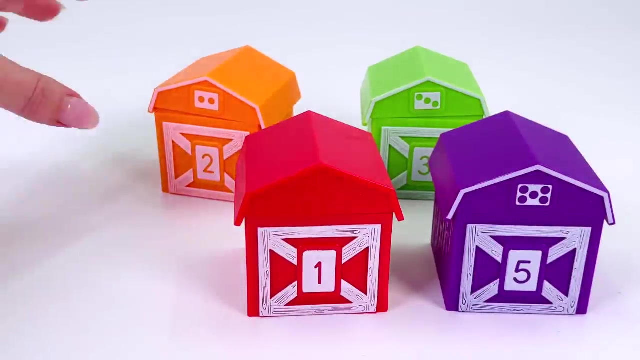 Wow, look at all the purple present. It says number nine on the front. I hear something And we found another number, The number nine. Let's put it back in the puzzle. Nine, Oh, what's this? Five barns. 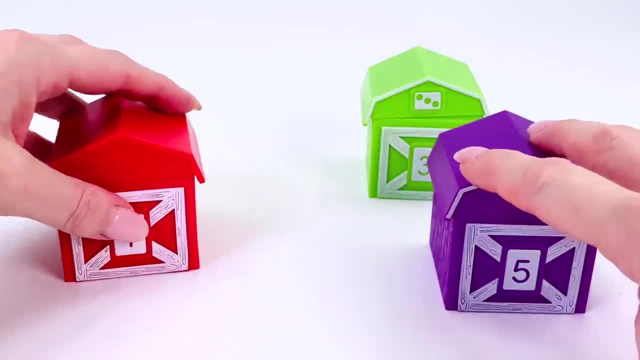 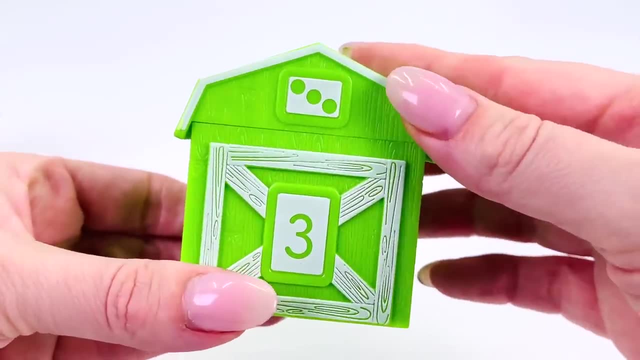 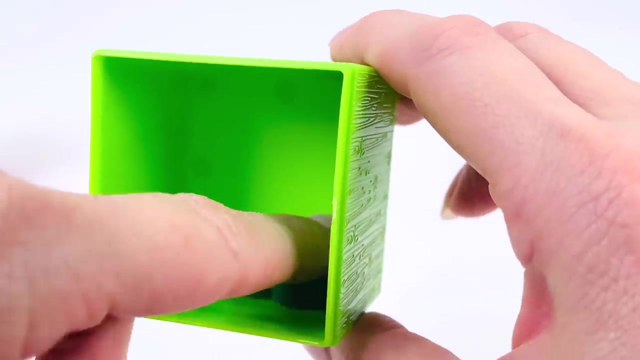 Hmm, Move this one over here and that one over there. How about we look inside barn number three? It's got a three on the front and three dots. Let's open the lid, Oh, and look Inside. the barn is number three. 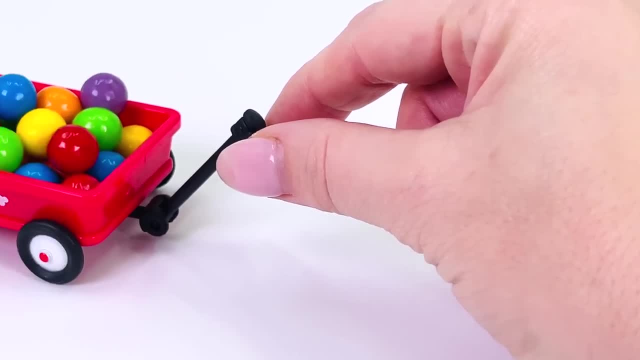 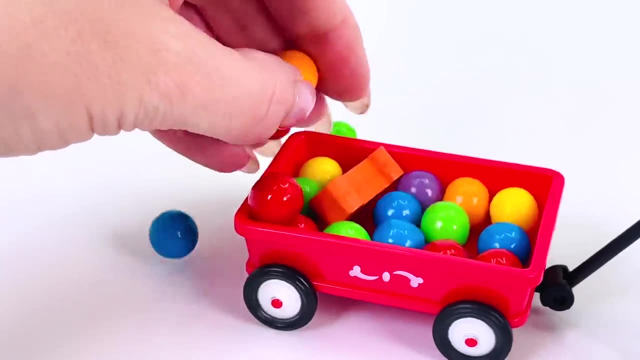 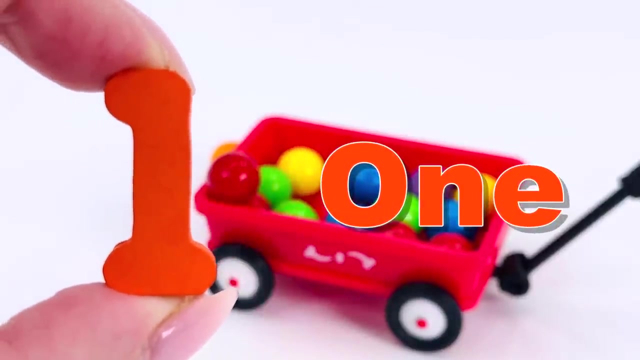 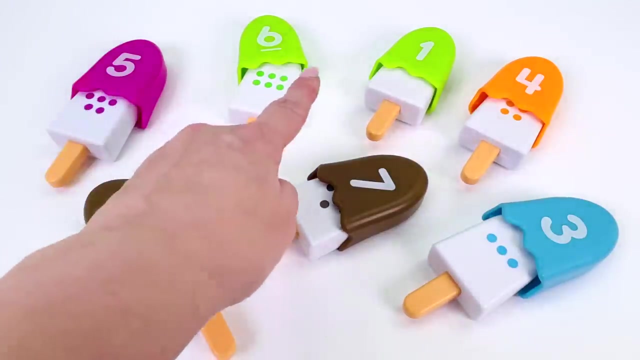 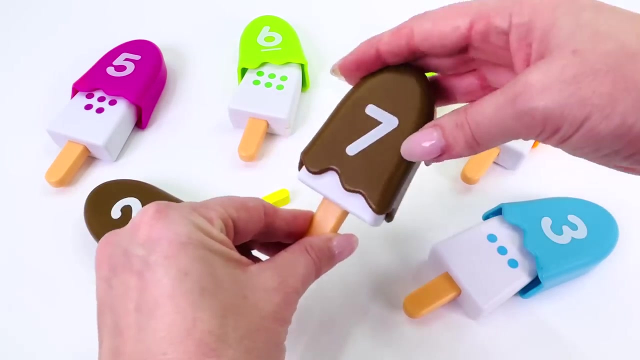 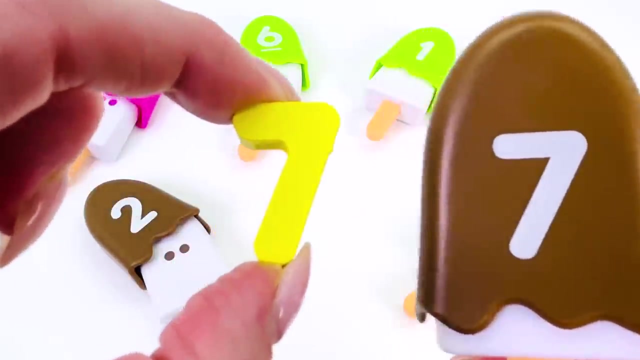 Three. Oh, it's a cute little red wagon. We found another number. We found the number one One. Look at all these number popsicles. Hmm, What one shall we? Ah, how about this one? Number seven. And look, There was a number seven hiding inside the popsicle. 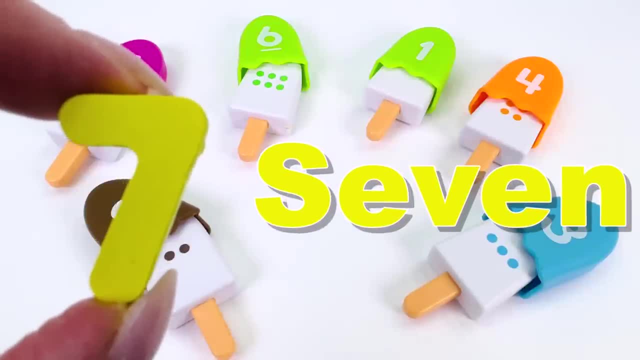 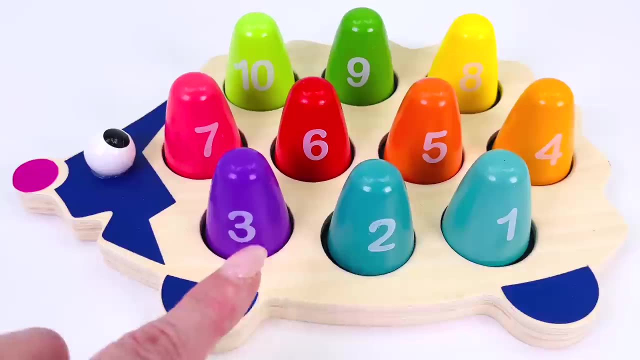 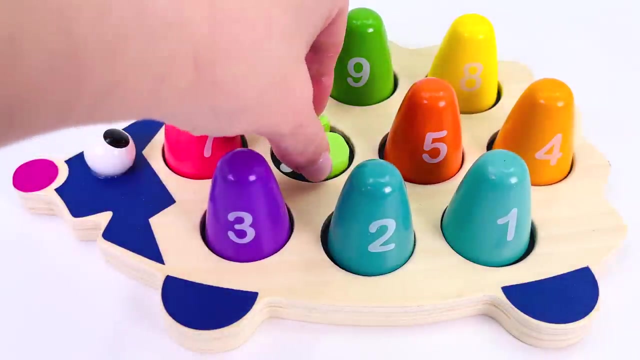 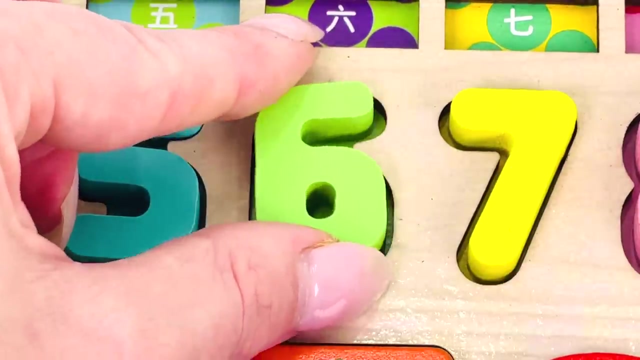 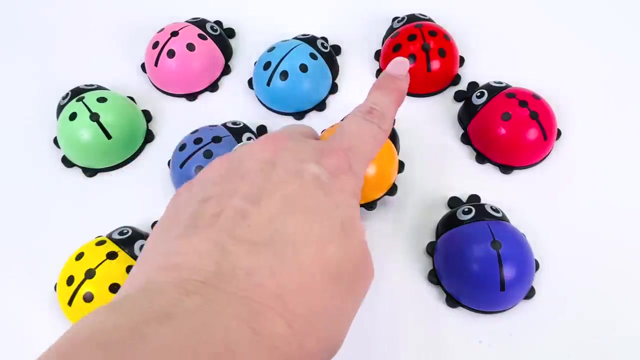 The number seven. Seven, This hedgehog has lots of spiky things. Hmm, How about we look under here, The number six. And we have our next number, The number six. Look at all the ladybugs. Hmm, I wonder where the number is hiding. How about this one, the orange one? 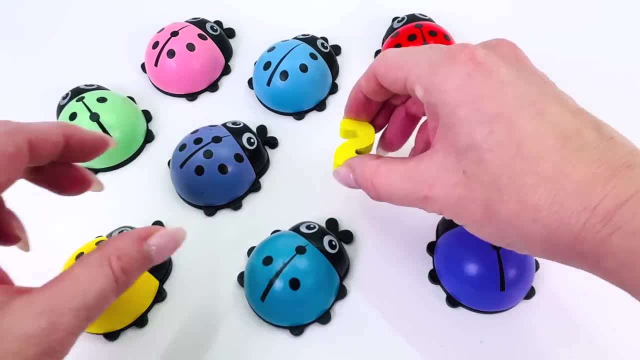 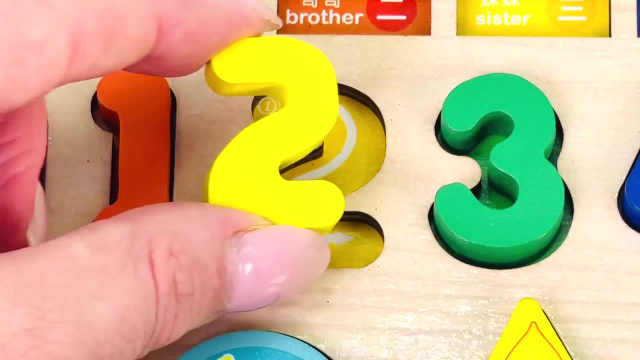 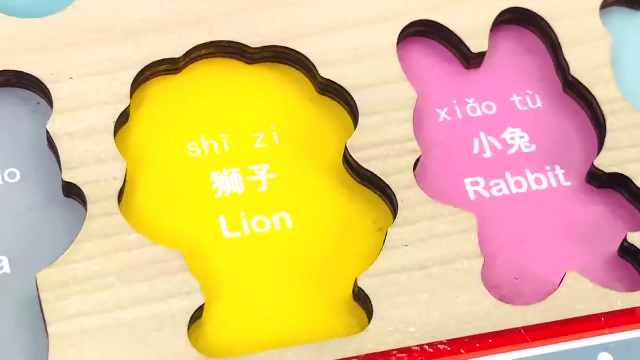 It has two dots And look, It has the number two underneath The number two. Let's put it back in the puzzle. Can you help me find all five animals? Okay, let's go look for them. Oh, the animals are all jumbled up. 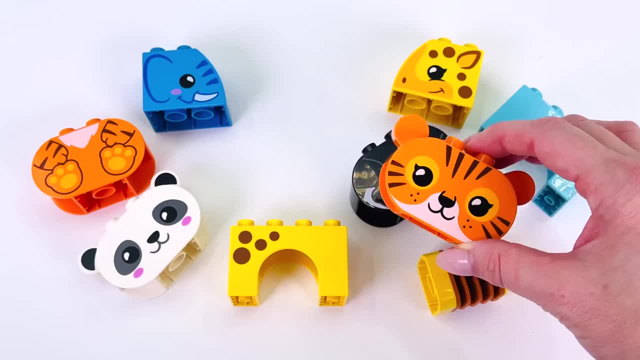 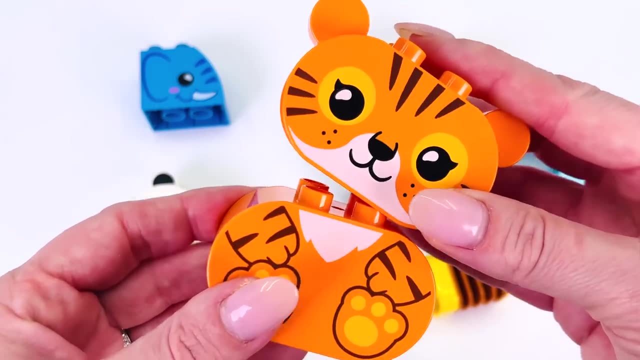 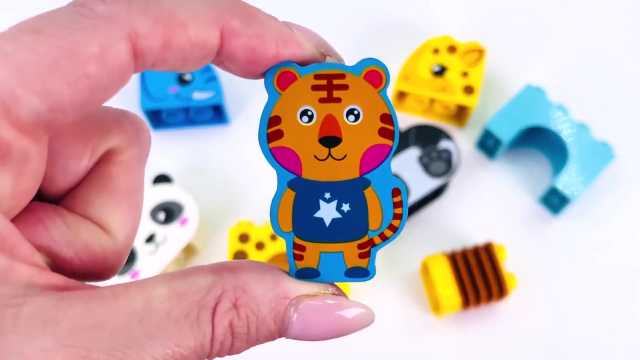 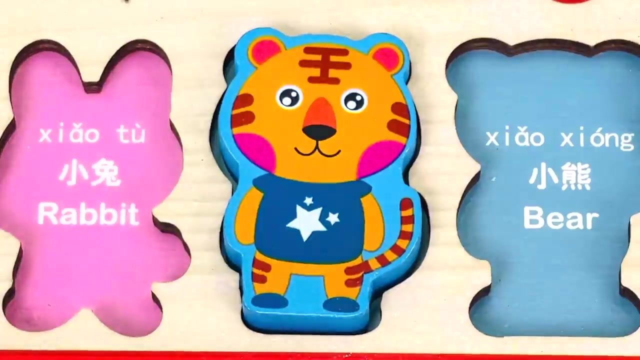 How about we make the tiger? I have its face. Can you see if you can find the body? Ah, here it is. It works. We made a tiger. Oh, and here's our puzzle piece: the tiger. Let's put it back in the puzzle Now. what shall we make next? How about the? 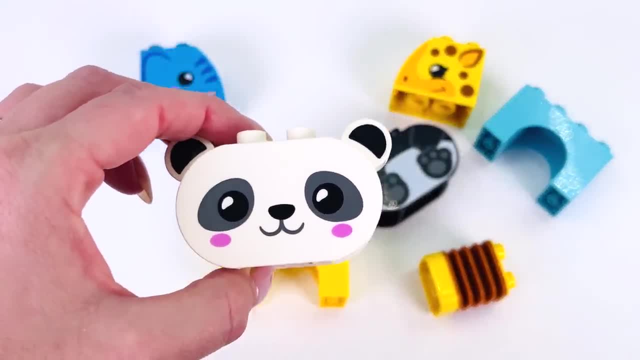 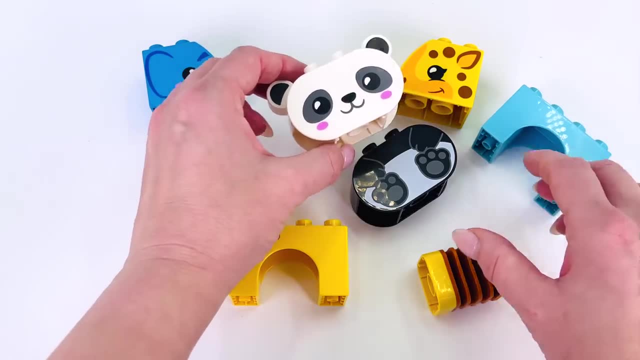 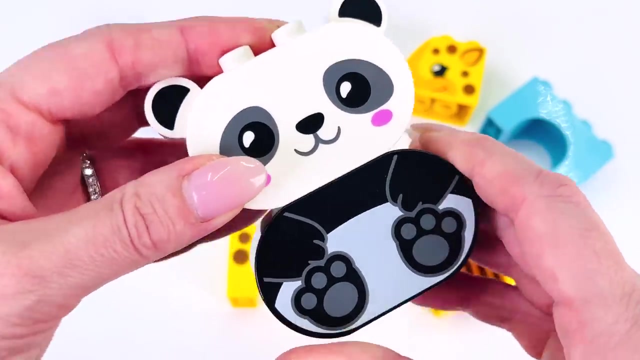 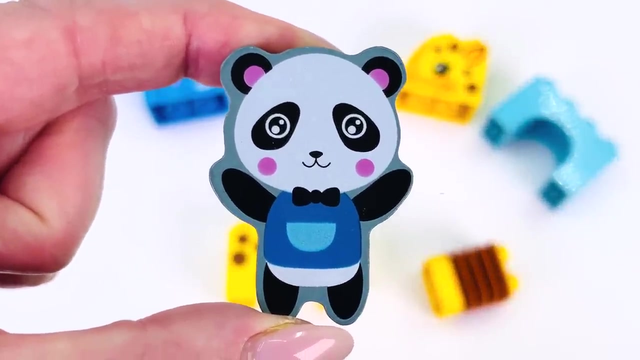 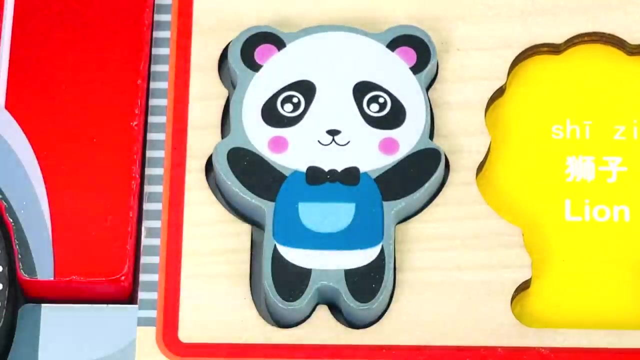 panda. Can you help me find the other half to the panda? It's the color black. Here it is. Let's put it together. We did it. We made a panda. Oh, and look, We have another shape, Panda. Let's put it back in the puzzle where it belongs. Can you help me find the lion? 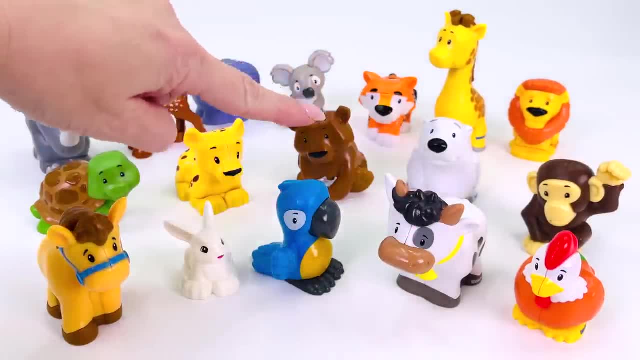 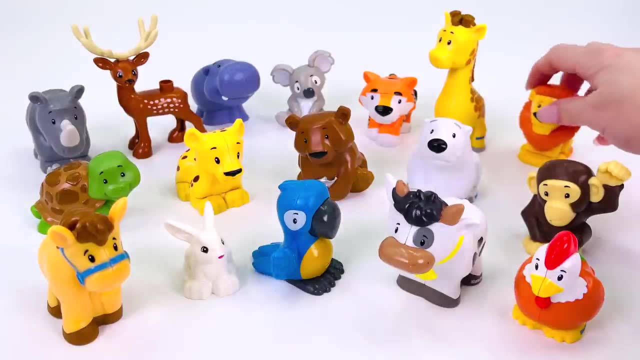 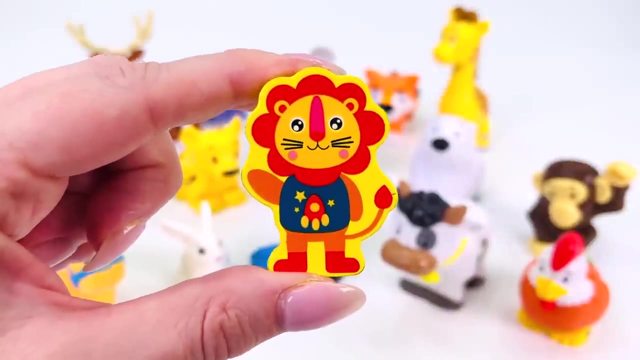 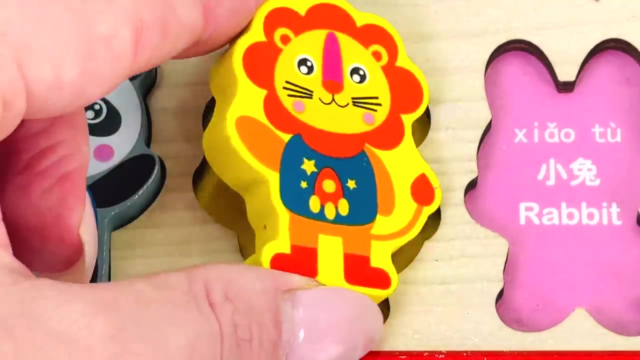 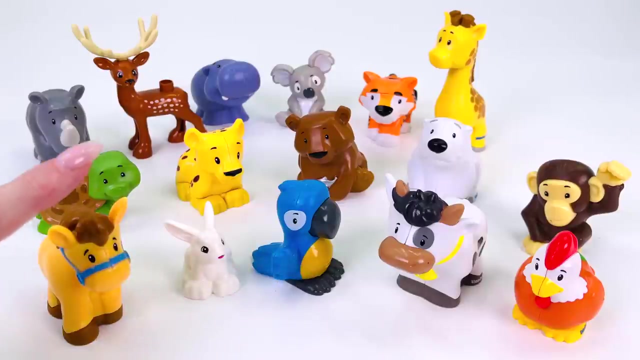 Not here, no, Not along here. How about this out over here at the back? yes, we did it. we found the lion. and look, we found another shape lion. now can you help me find the brown bear? it's not here, no, not up here. oh, where is it? oh, here it is in the middle. 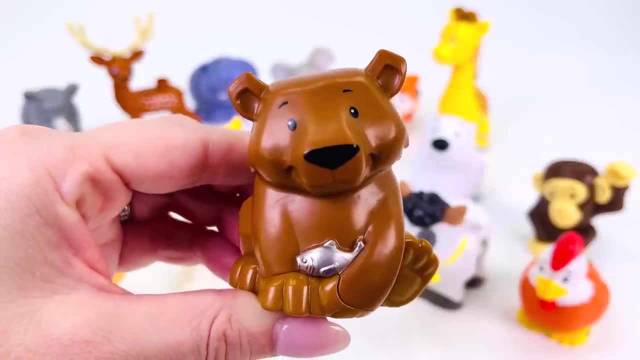 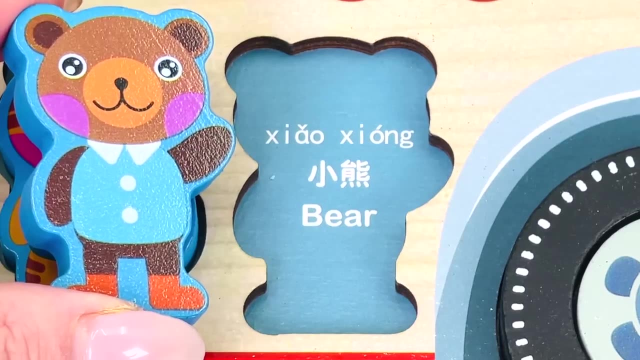 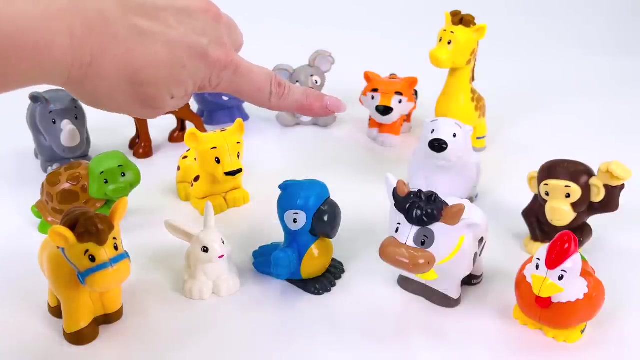 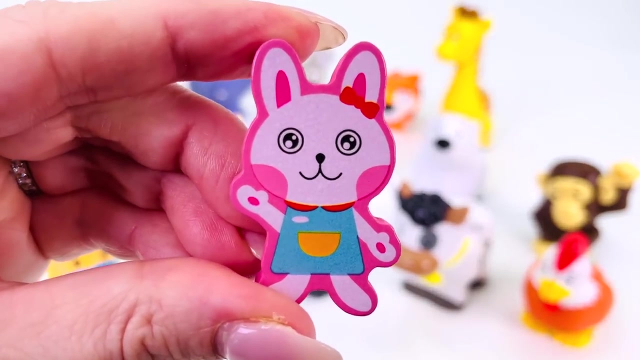 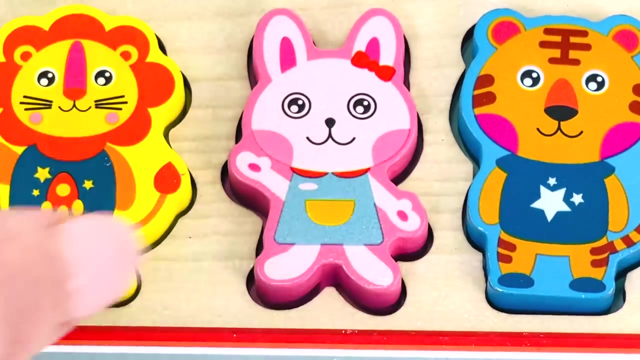 we found the brown bear, oh, and it's turned into a shape bear. now can you find a white rabbit? it's not up here, not here. oh, here it is. we found it and look, we have another shape. it's a rabbit. let's put it back in the puzzle where it belongs. great job. now can you help me? 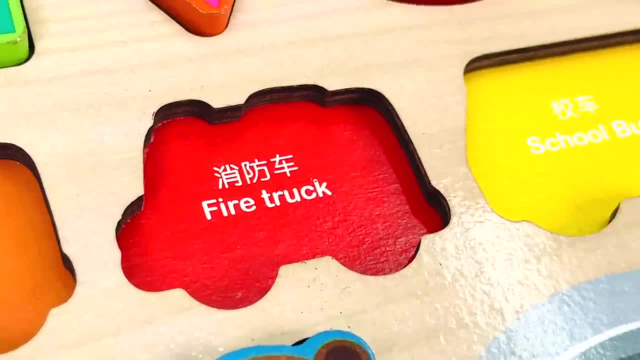 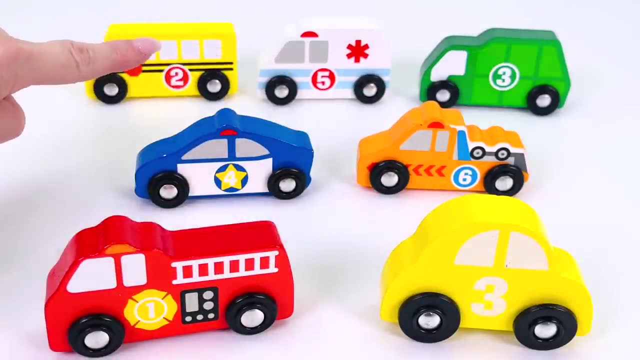 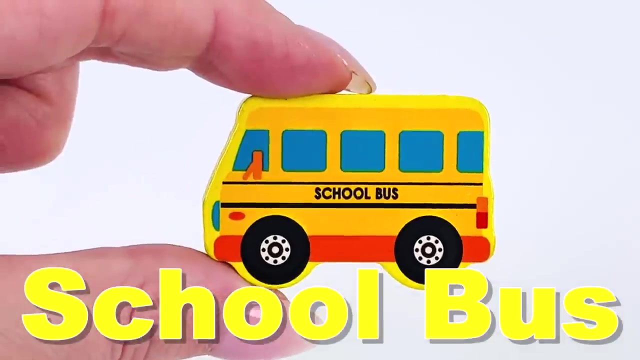 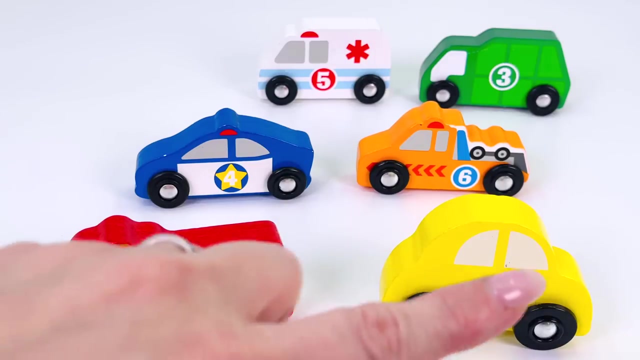 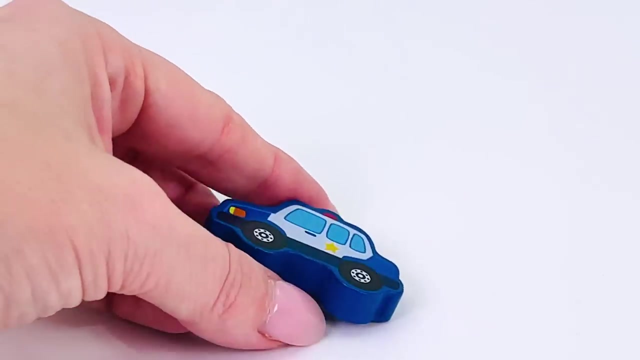 find all five vehicles. I need to find the school bus. can you see the school bus here? it is right here, school bus. oh, it's turned into a puzzle piece. a yellow school bus. can you find the blue police car? not up here? it's over here. it's turned into a puzzle piece. the police car. 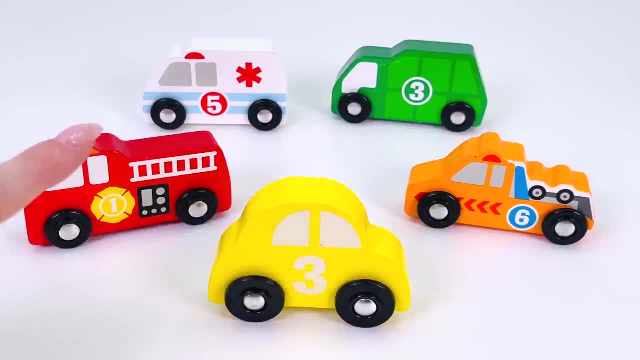 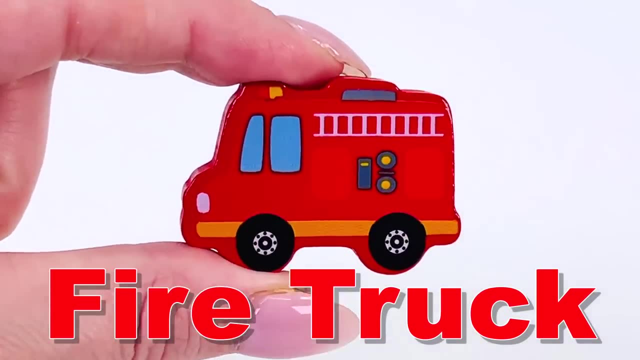 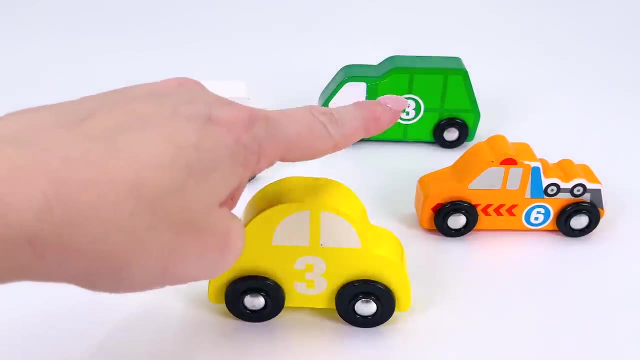 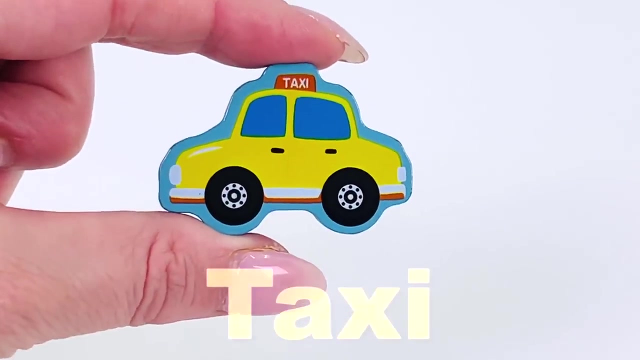 next? I need to find the red school bus. what's next? what about the fire engine? here it is, and we have our next puzzle piece: the fire engine. what's next? how about the taxi? here it is. we found a little yellow taxi. let's put it in the puzzle. we only have one last vehicle. 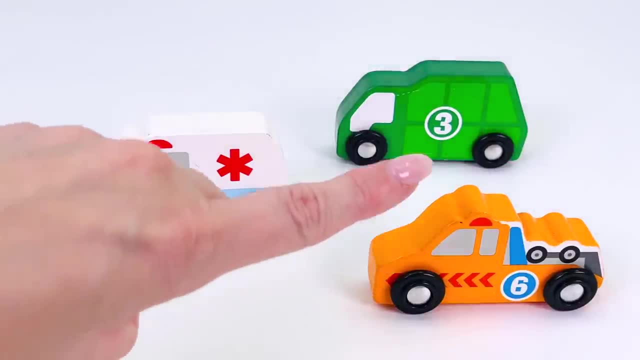 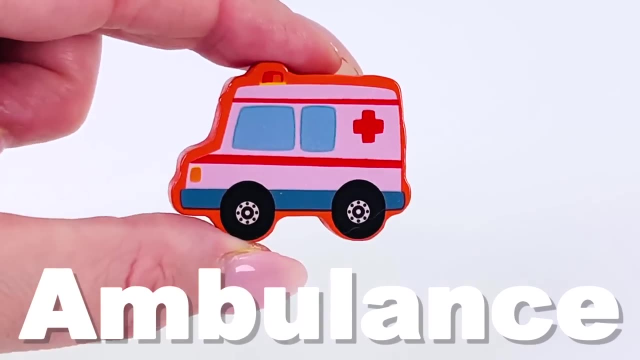 oh, here's the yellow taxi. we need to find the yellow taxi. lets put it in the puzzle. we have a little yellow next to the yellow taxi, so we're gonna put this away and we'll call back the fire engine, fire engine- to find the ambulance. ah, here it is, and we found our last vehicle. puzzle piece. 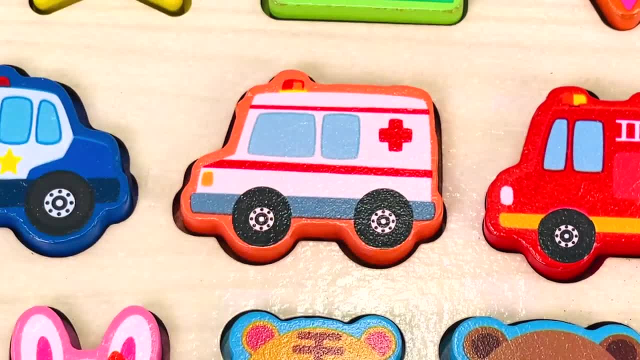 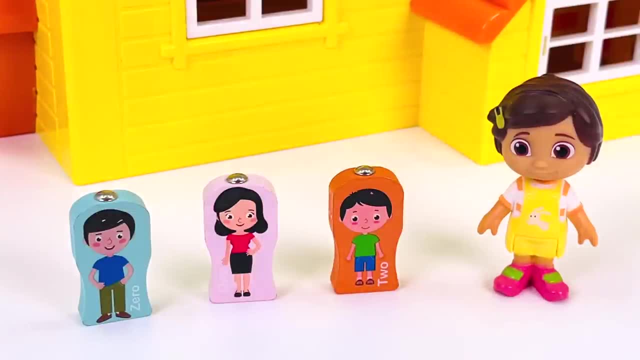 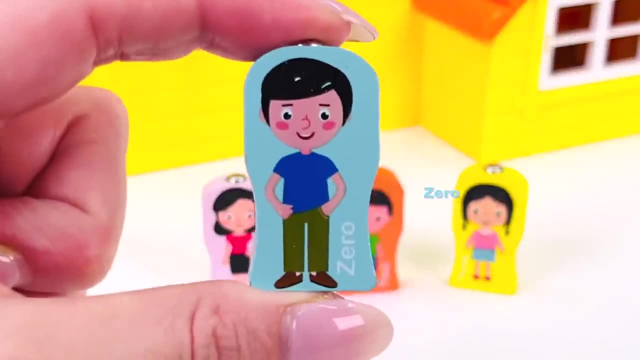 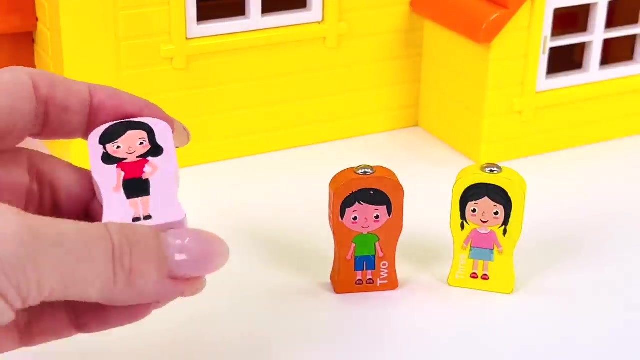 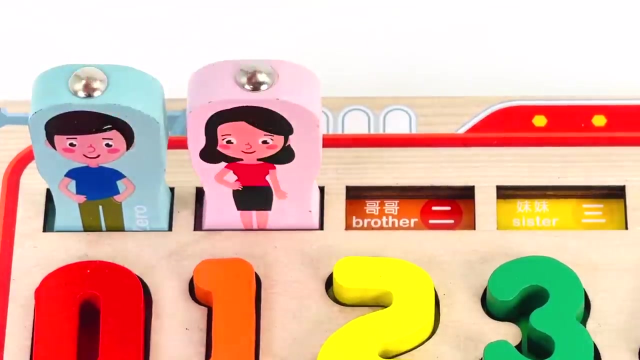 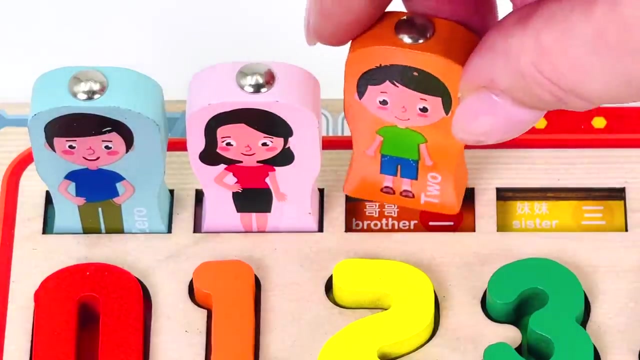 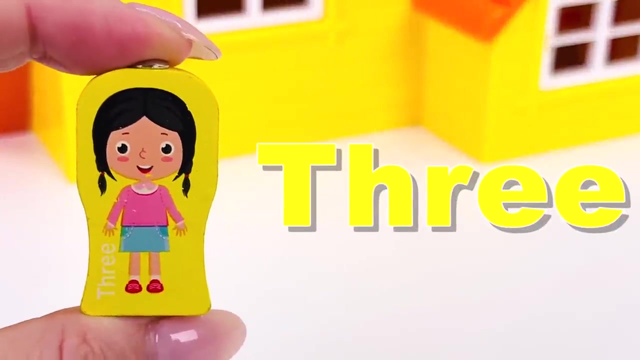 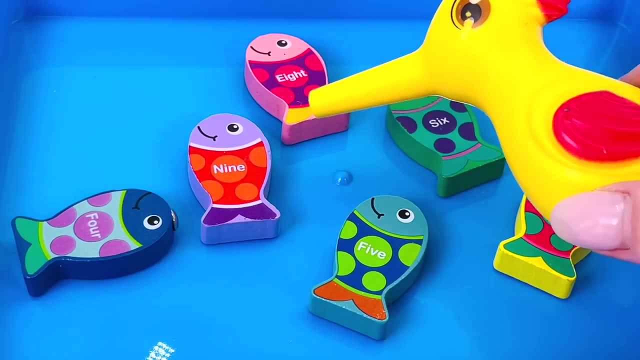 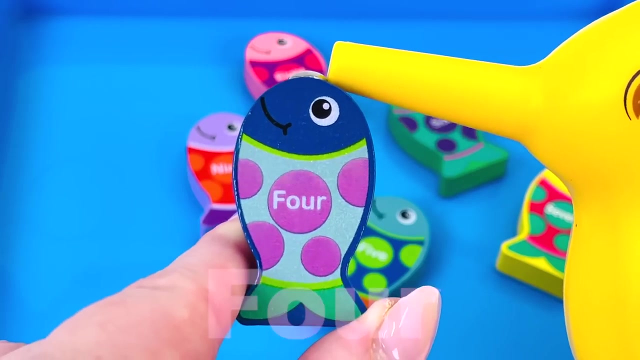 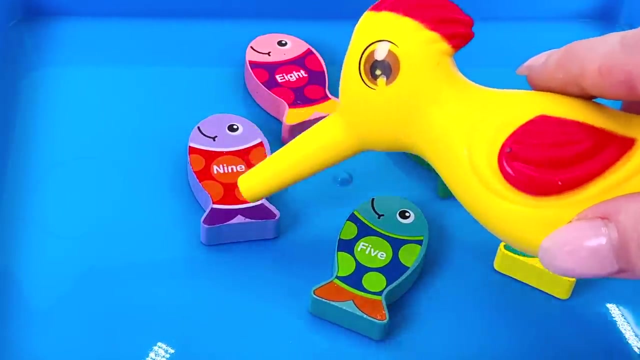 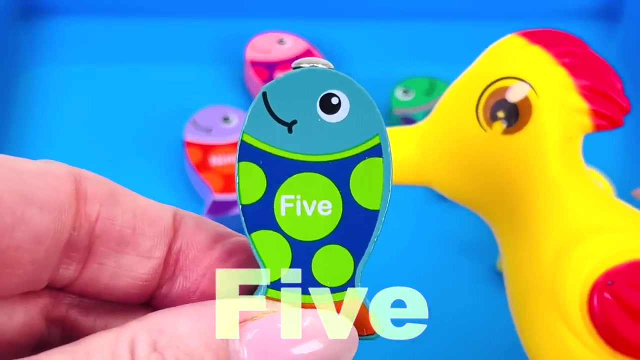 the ambulance. great job, brother. brother, brother and sister. there's four more pieces to put in the puzzle. let's count them. it's zero, one, two, three. let's keep counting by catching fish. that's four. can you see number four? five, five. let's look for number six.